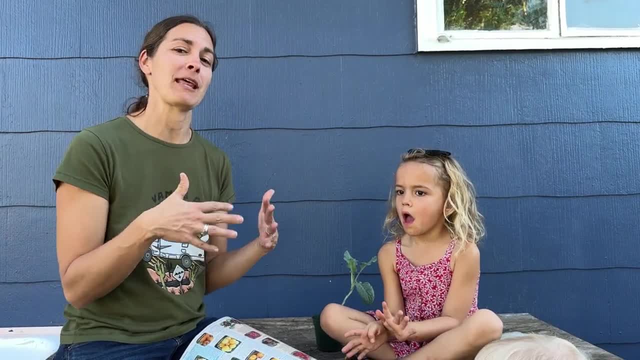 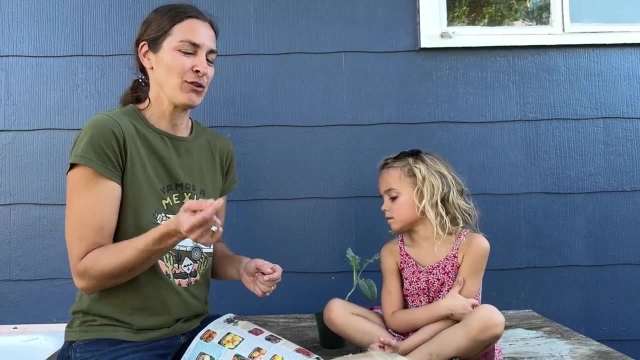 And then they are excited because they took ownership in that process and they annihilate the fennel And they'll surprise you so often because they chose it. They'll be willing to try it a lot more willingly if they had no say in it. So flip through seed catalogs. 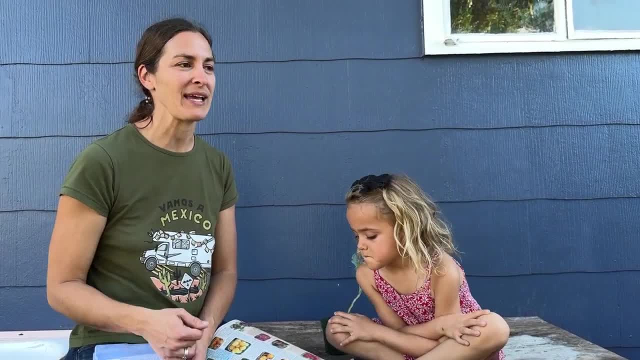 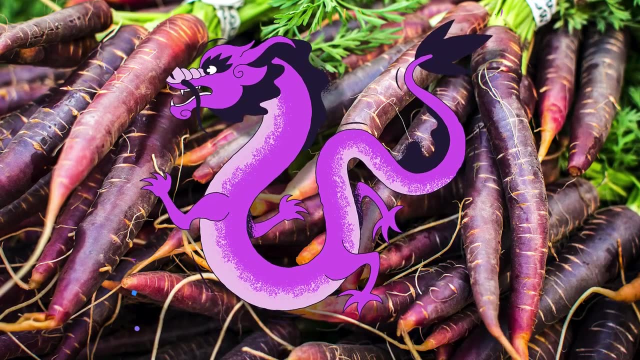 read descriptions. They like picking by name. So like the dragon- purple dragon carrots- I'm like, oh my gosh, I want to grow carrots. It's a purple dragon. What kid doesn't want a purple dragon carrot, right, Yum? 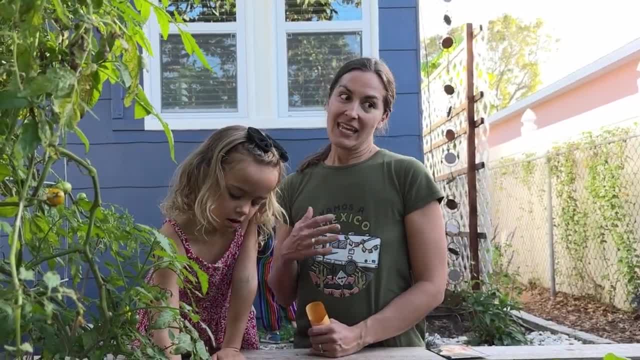 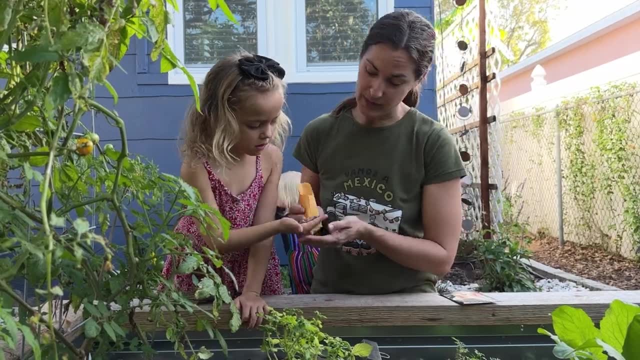 So, when it comes to actually planting in the garden, this is going to take practice and patience, So I've learned a few different ways to go about it when you're working with them, especially the first few times that you're in the garden. 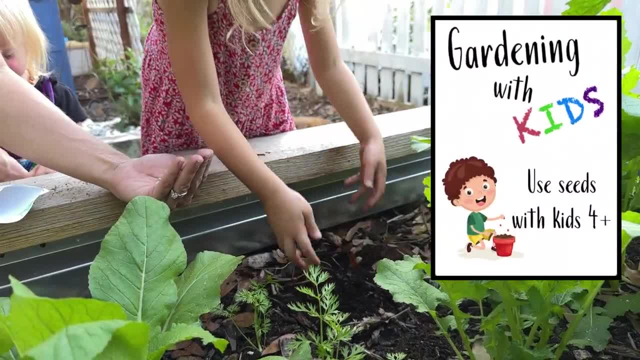 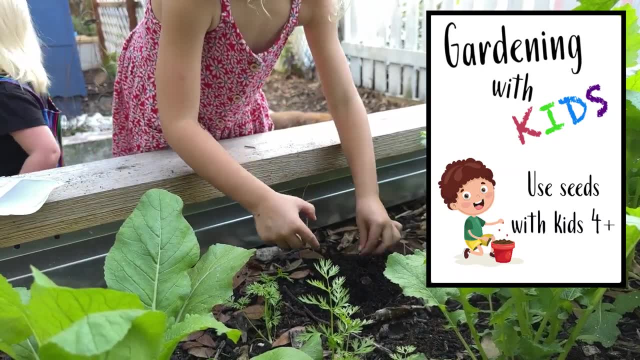 For kids four and up start with seeds. They do good sticking their finger in and planting the seeds, And then, if you're a little unsure about whether it's going to take, I will oftentimes just follow up afterwards and replant more seeds, so that you know that. 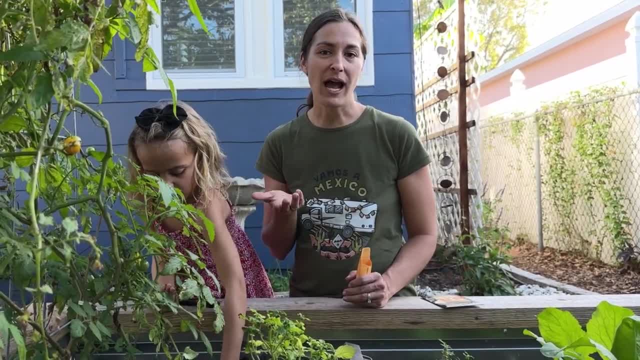 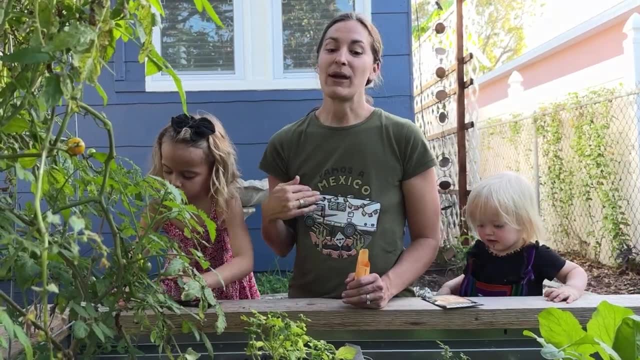 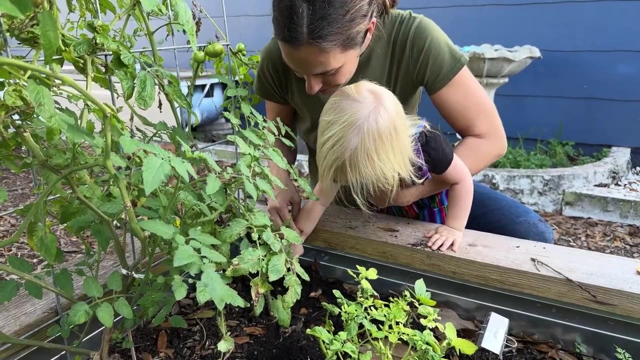 they will germinate. So if they buried them a little too deep or too shallow, I usually will just wait a little while and then go back and remedy the situation, So that way they can see where they planted it. And then the other thing that I found is with little hands, even when 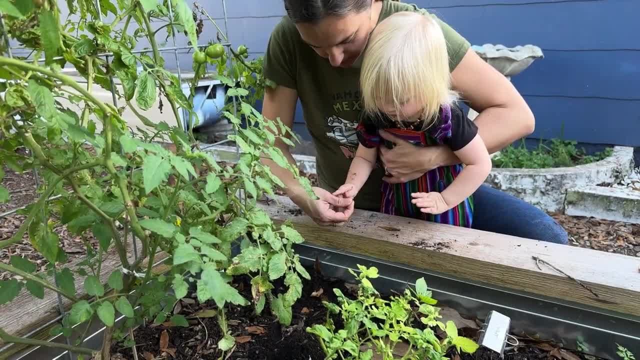 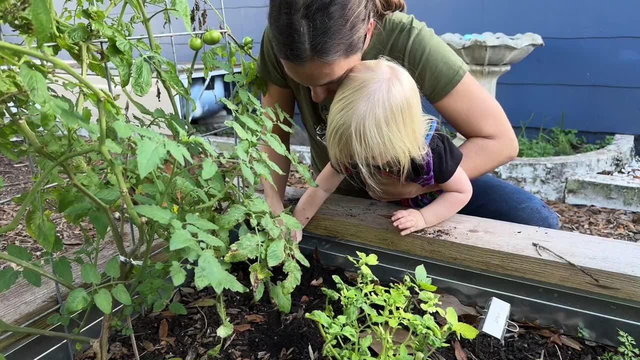 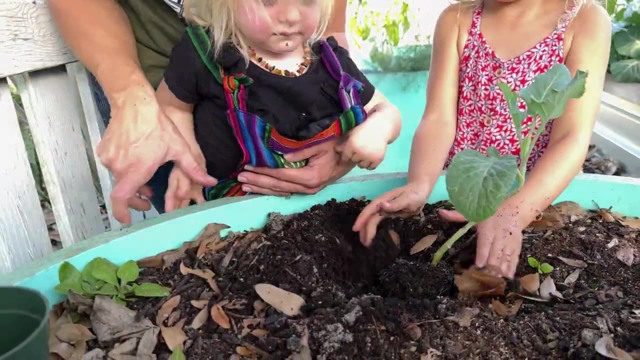 they're toddlers like this. larger seeds like peas or beans are easier for them to handle, So have them help with that, instead of lettuce or carrot seeds, which are super, super tiny. Their dexterity can handle that a lot better. And for the youngest ones, if they aren't getting the 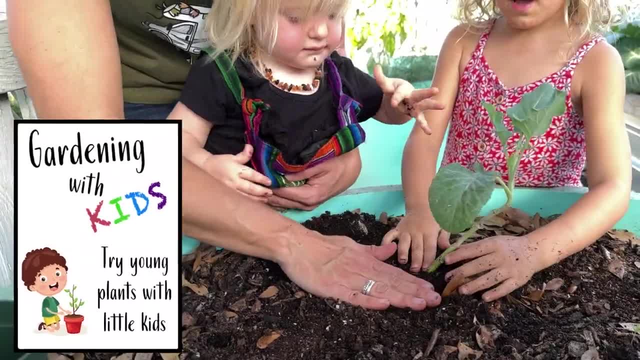 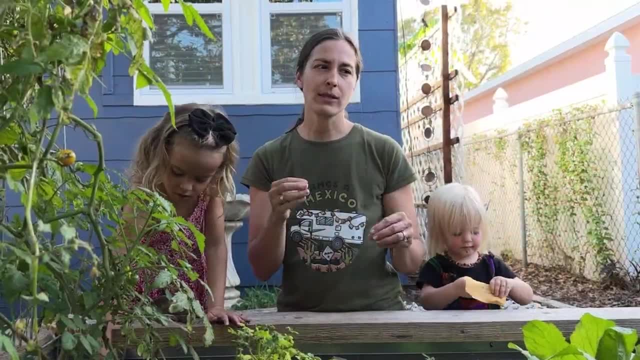 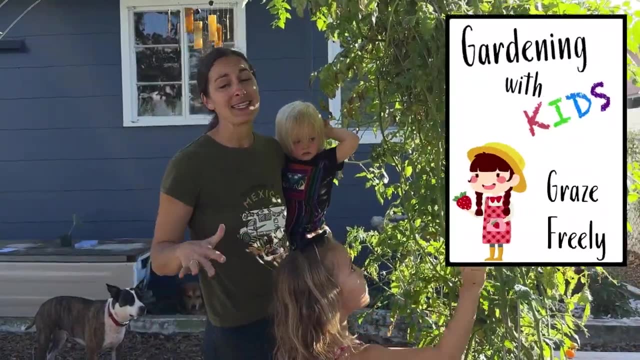 seed thing too well. you can always do live plants, Believe it or not, they do really well And if it comes down to it, digging a hole and having them plant the plant is a lot easier than them trying to understand and navigate planting a seed. So one thing that's really important is to graze freely. 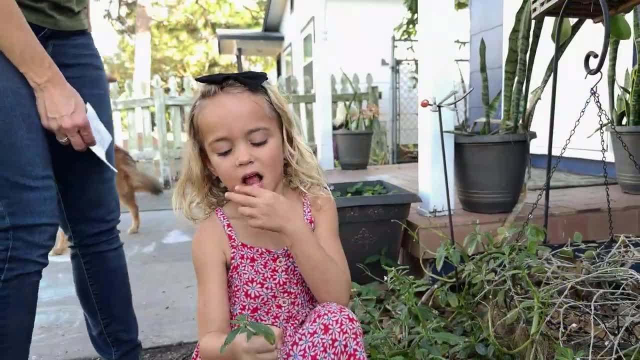 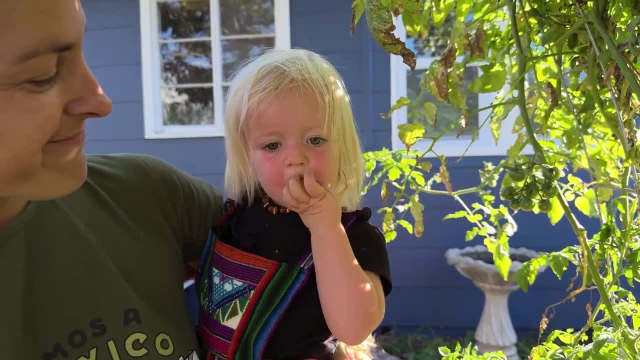 even if you were planning on using it for a recipe or you weren't really intending on picking it quite yet. letting them graze it with abandon and just freely Like if they're interested in eating something, let them. I remember the first time Layla ate a carrot. We picked it out of the 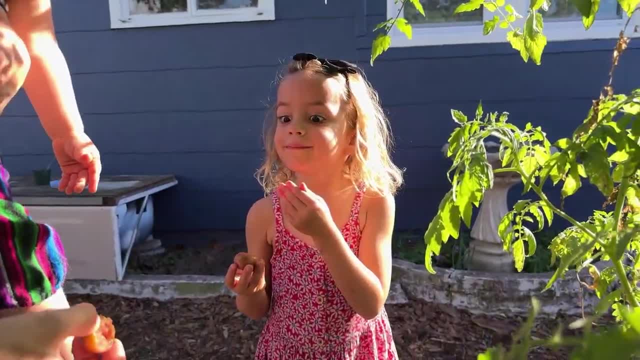 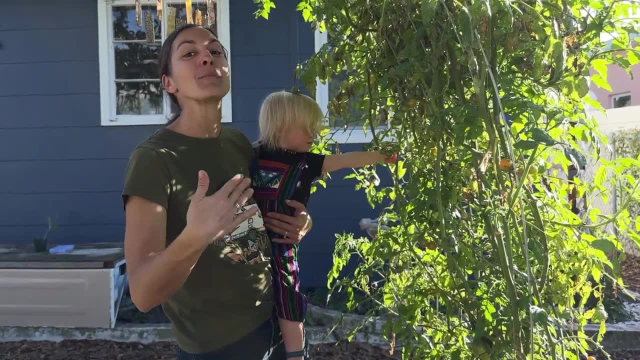 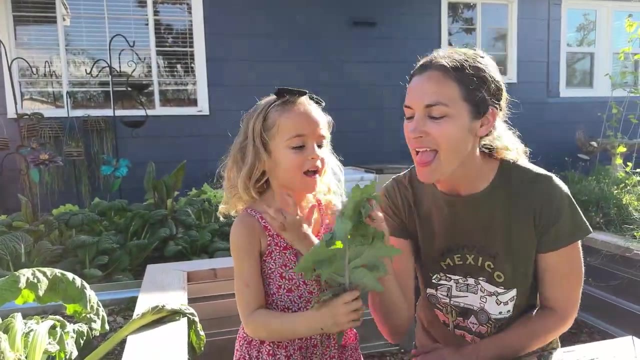 garden together and she was so excited and she goes to eat it. no rinsing nothing, it's covered in dirt- and i went to go grab it out of her hand and then i was like you know what, like this is the moment we're working to recreate, so just let them eat, um, enjoy it and graze with them, them seeing. 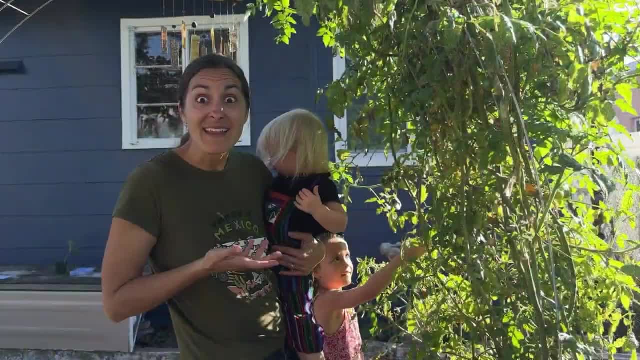 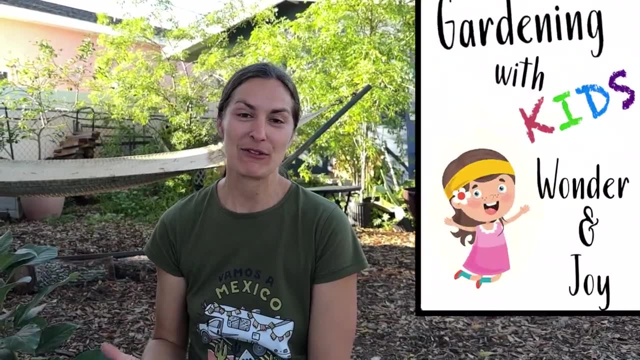 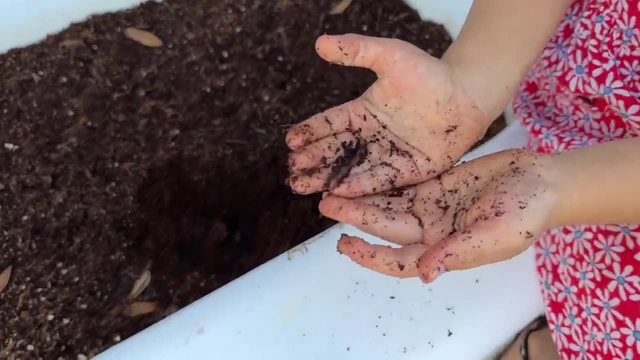 you do the same thing shows them that it's okay and that it's acceptable. so pick freely and enjoy. children are full of wonder and joy, whether it's chicken eggs or pests or flower blooms, or how amazing it is that the tomato goes from green to red, showing wonder and joy. 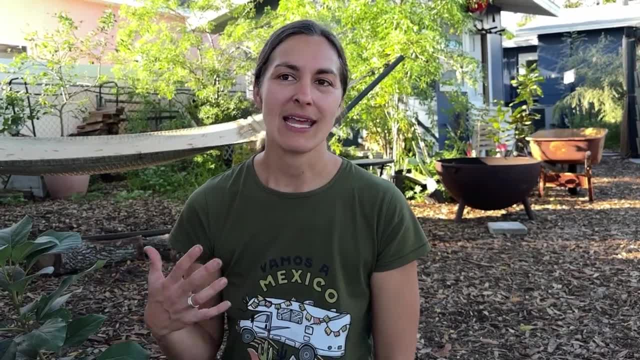 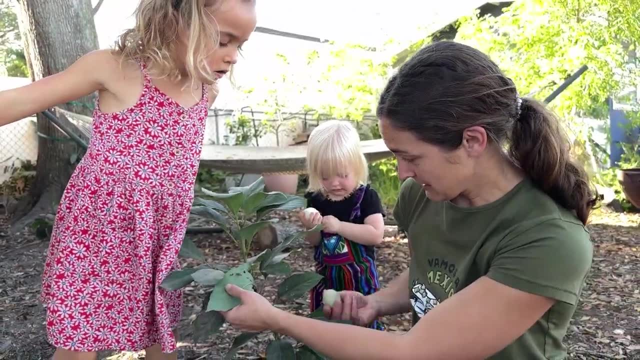 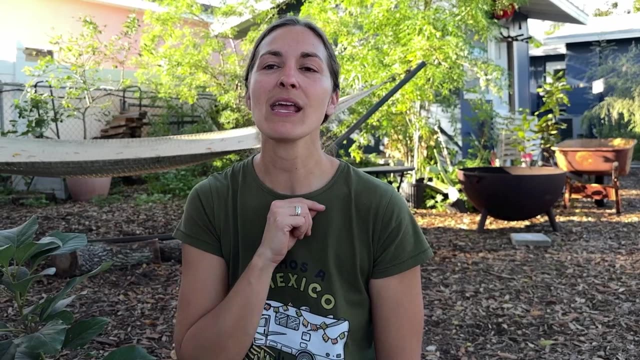 and pure amazement at the natural world is what really can help them connect as well as us. i've also never seen my plants so caterpillar free. when i shared the fact that things love caterpillars, they went out daily. every time they got out in the garden they would. 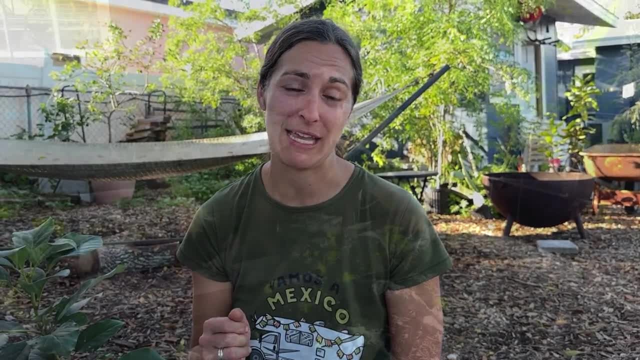 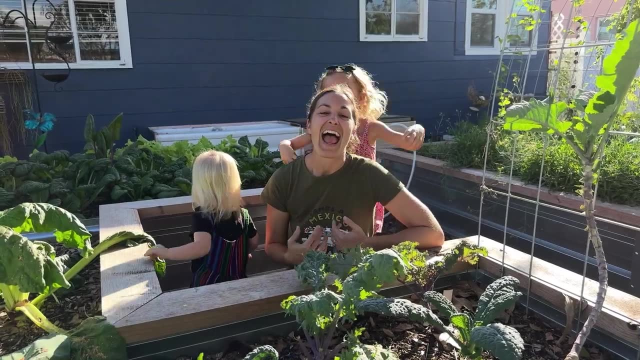 run over to the plants, flip over the cucumber leaves and start looking. one thing that we have to remember when working in the garden is that we are working with children and they're kids and they're going to be kids. so we have to have a little acceptance, a little bit of patience. 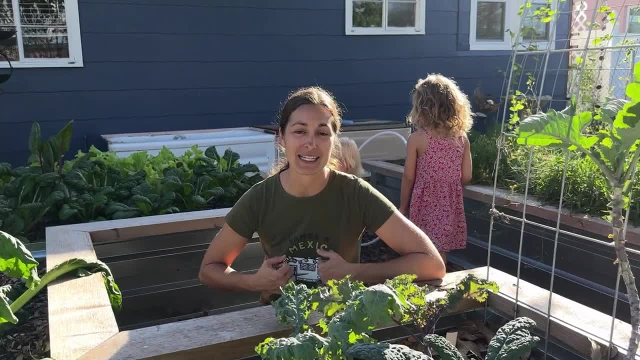 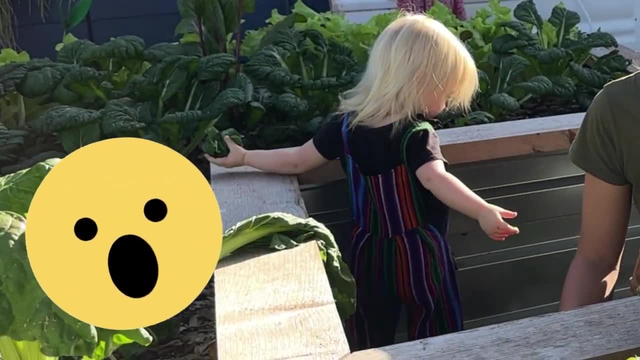 i work at her farm school and i cannot tell you how many times the kids come running up to me with in their faces and an entire plant, because they picked the plants when it was ready. I don't think we will ever get a carrot to come to full size at the school, but that's. 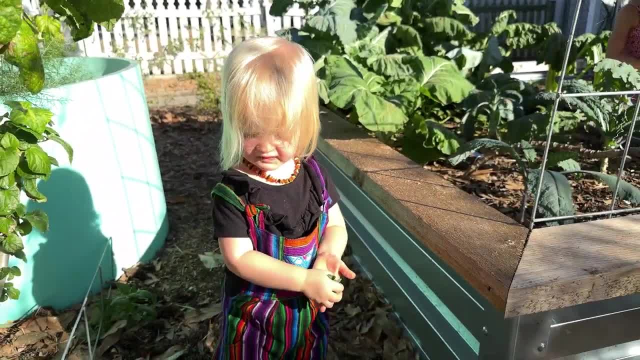 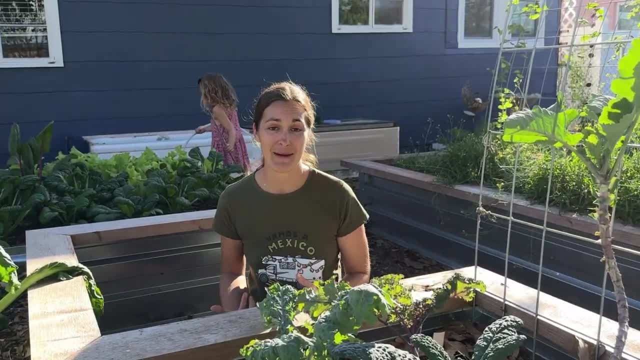 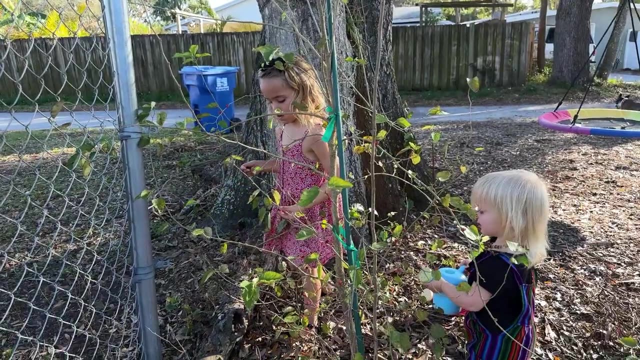 not the point. The point is to get them involved and enjoying their time in the garden. So lots and lots of patience for yourself and with them. Every time they come running up to you with something you might not have wanted them to harvest, just a kind, gentle breath and reminding them how we harvest it. 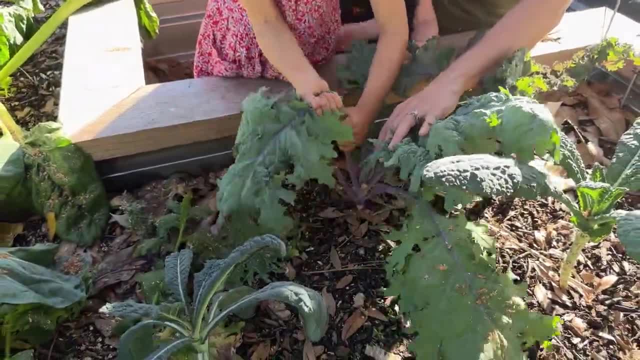 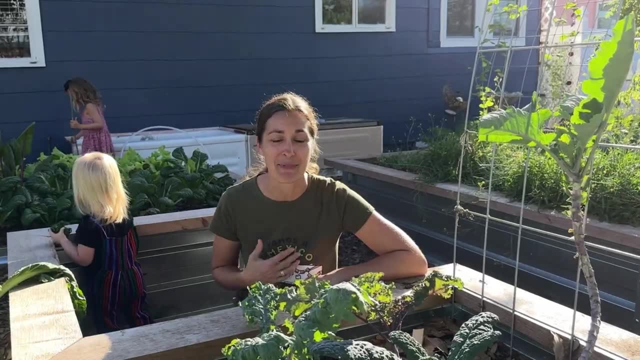 We hold the plant and then we break the stem. We wait until they're red, not green. These will become repetitive patterns in the garden, but repetition is key for children. So I've been with my own children in the garden since they were born.